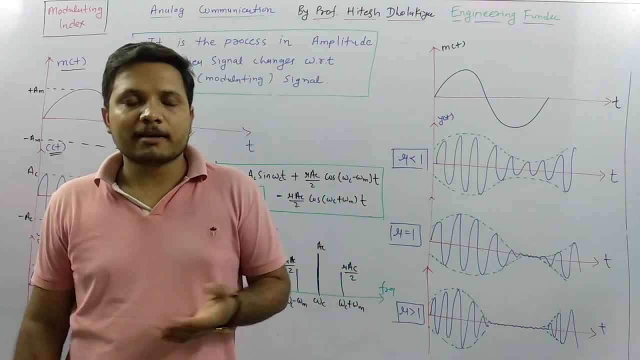 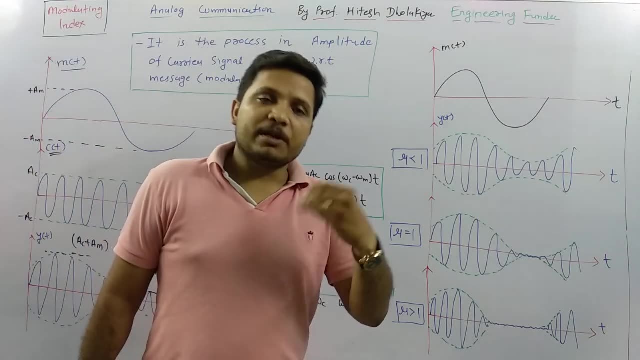 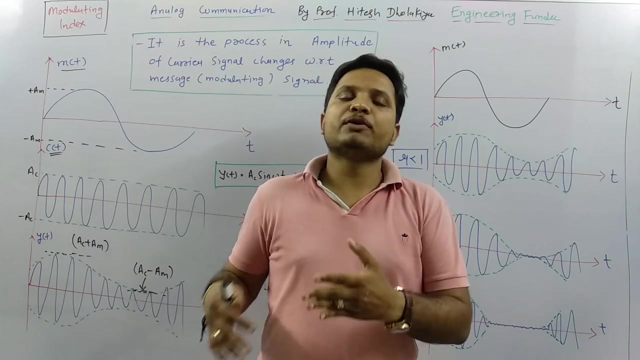 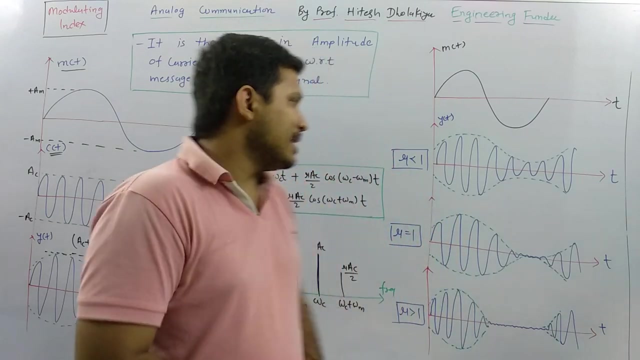 Welcome to communication engineering playlist. Here in this session I will be going to explain modulating index in amplitude modulation. Now, see in previous session I have already explained you what is amplitude modulation and based on that we have derived amplitude modulated signal. Now in that amplitude modulated signal, if you have remembered that derivation, 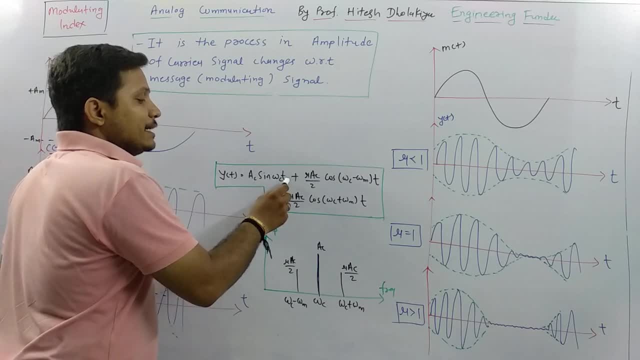 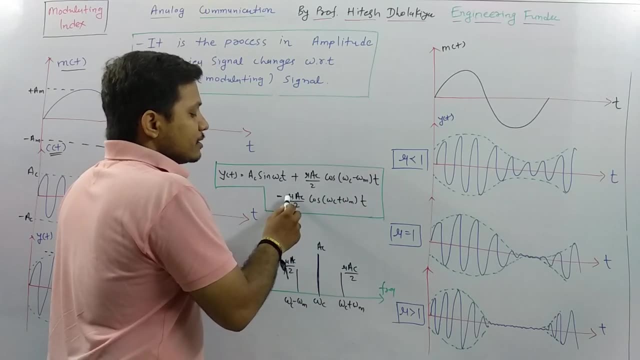 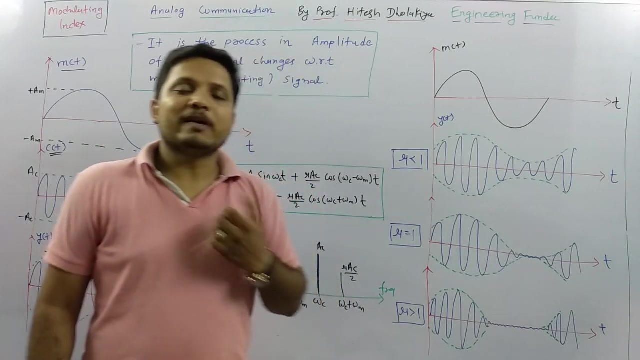 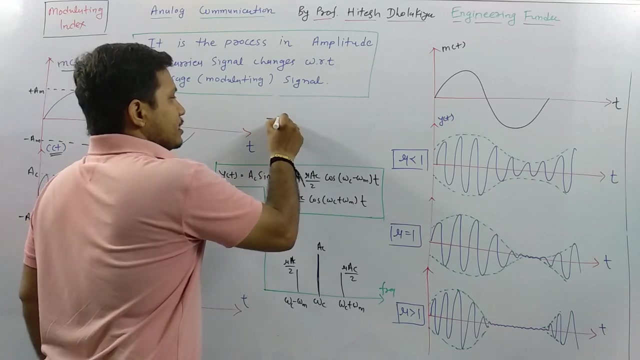 was y t is a c sin omega c t plus mu a c by 2 cos of omega c minus omega m t minus mu a c, by 2 cos of omega c plus omega m t. So that is what the basic equation which we have derived in last session, Now here: mu, that is modulating index, mu, that is modulating. 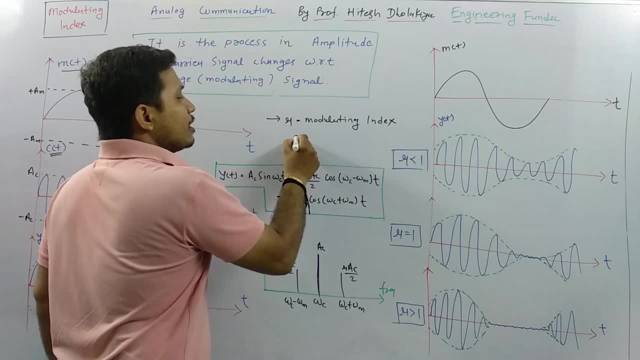 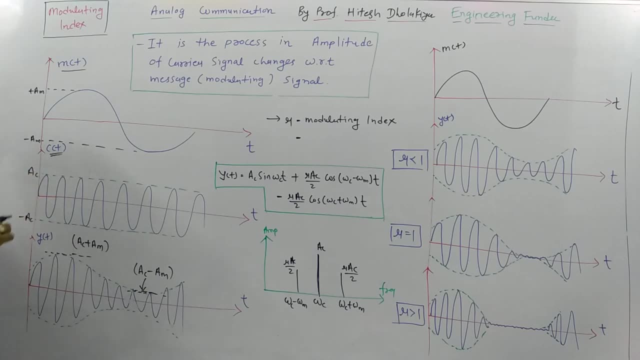 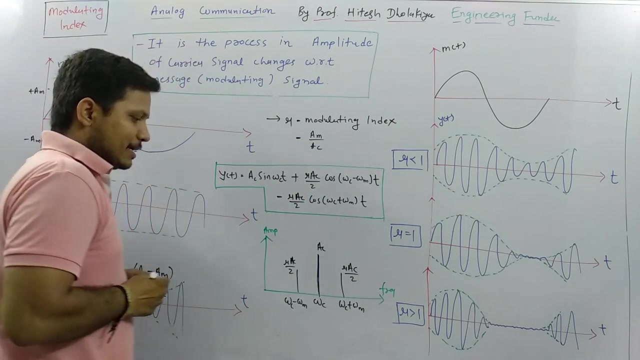 index and that modulating index is amplitude of modulating signal divided by amplitude of carrier signal. So here, amplitude of modulating signal, that is a m and amplitude of carrier signal is a c. So modulating index that is a m divided by a c. Now, as I have told you, 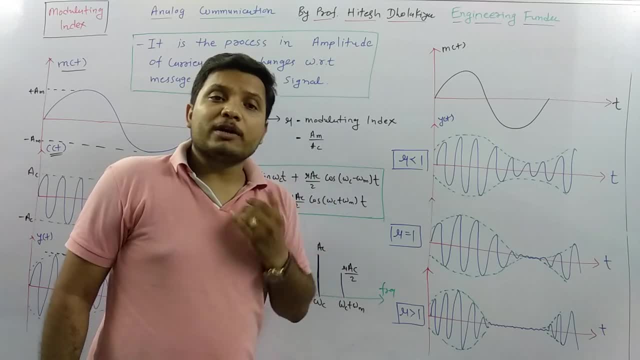 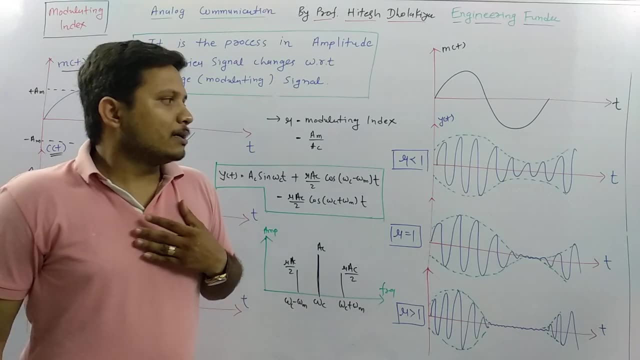 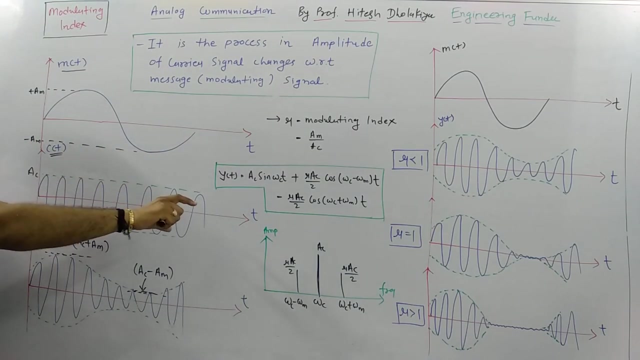 in last session, like modulating index. Modulating index plays very important role in amplitude modulation, So I have made this separate session for understanding of modulating index, Like see, as I have explained you, if you have input signal like this and carrier signal like this, which is high frequency carrier, 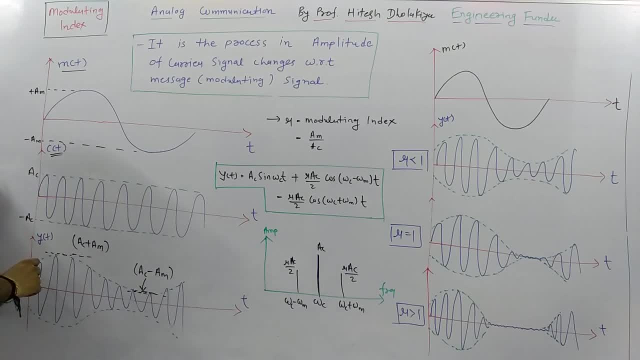 signal compared to modulating signal, Then in amplitude modulation output signal will vary with respect to modulating signal where amplitude of carrier signal is equal to amplitude of carrier signal. So in this example output signal of carrier signal will vary with respect carrier signal is getting change, so carrier signal amplitude that is getting change. and 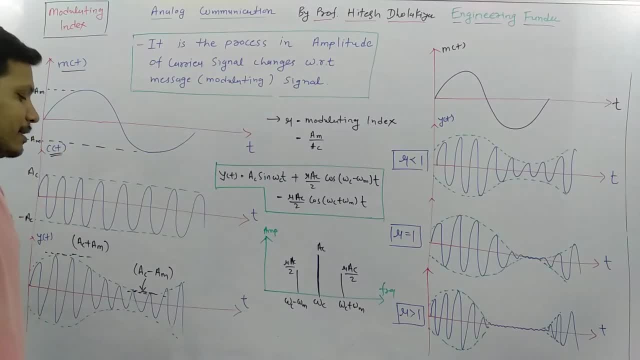 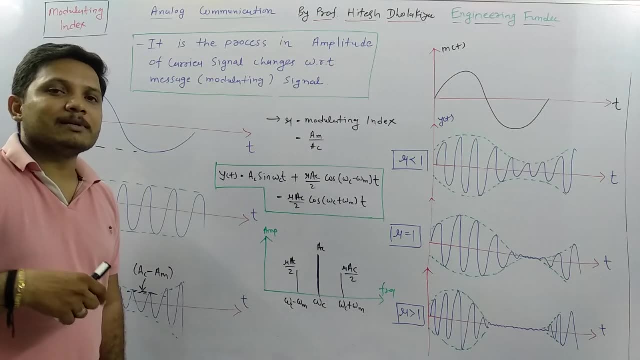 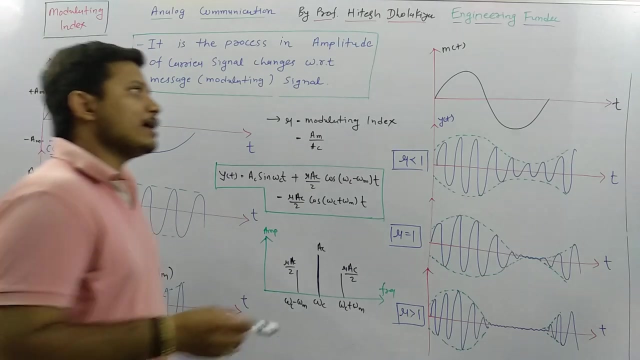 if you see that derivation where mu is am by ac. so, as i have told you, mu modulating index that should be lower than unity. otherwise there is a possibility that we can have phase distortion. so that i will explain like: see, here i have modulating signal and that modulating 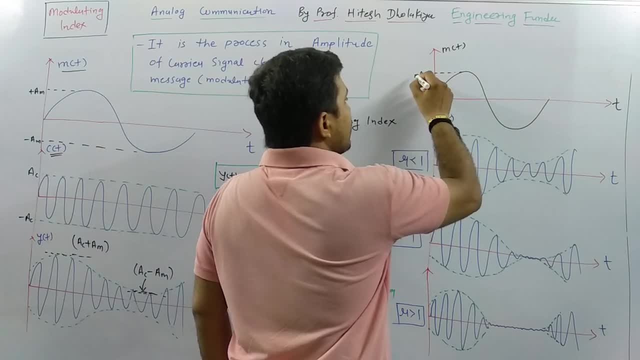 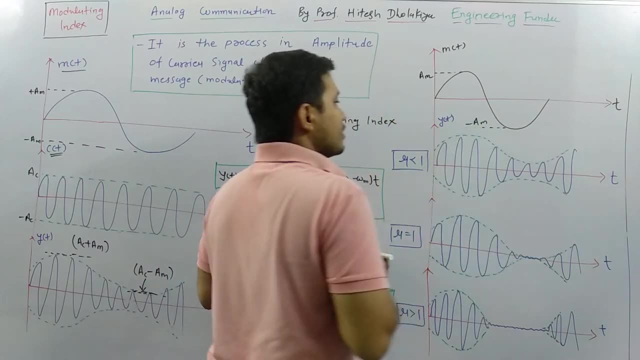 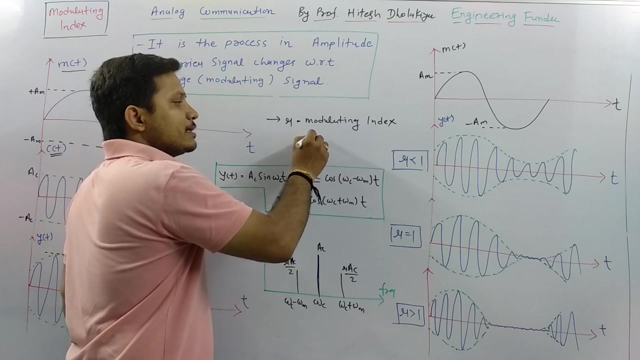 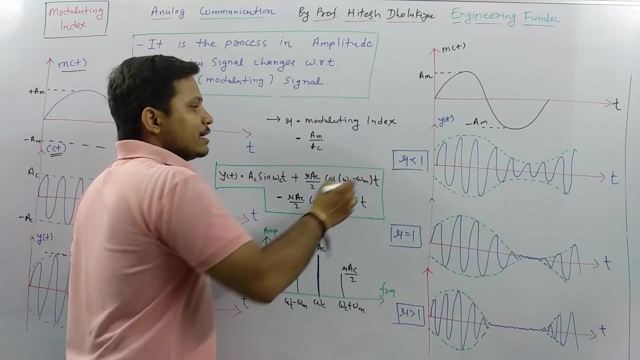 signal that is having amplitude varies from plus am to minus am right. so here this amplitude is minus am. now, if i have modulating index that is lower than 1, it means am. by ac that is lower than 1, it means am is lower than ac. so if modulating index that is lower than 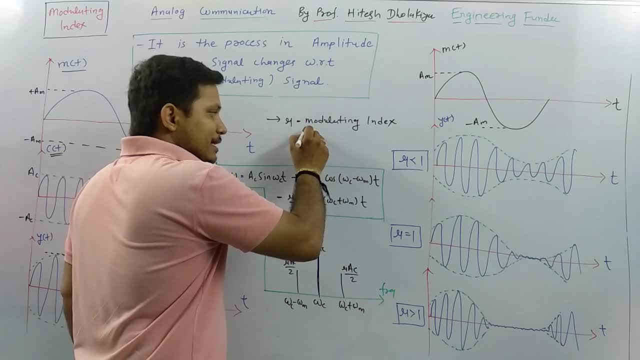 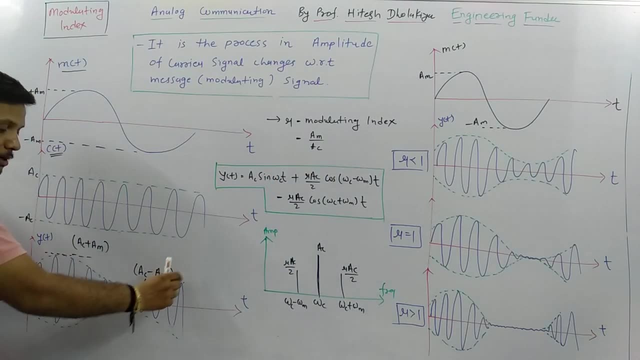 1 means modulating. modulating signals amplitude is less than carrier signals amplitude. so, as you can see, this modulated signal that is having maximum amplitude, which is ac plus am, and minimum amplitude that is ac minus am. so here what will happen? this minimum signal that is ac minus am, where, if 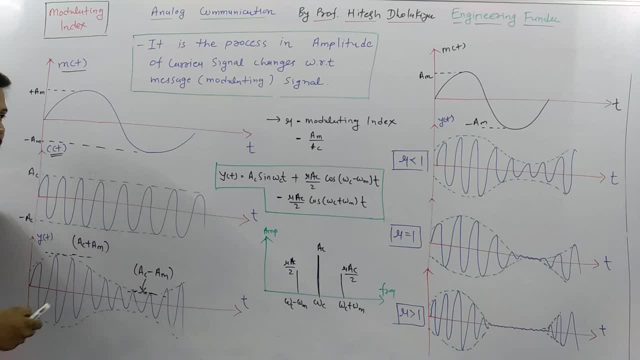 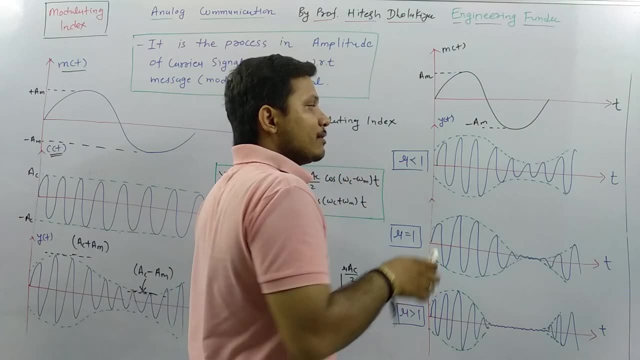 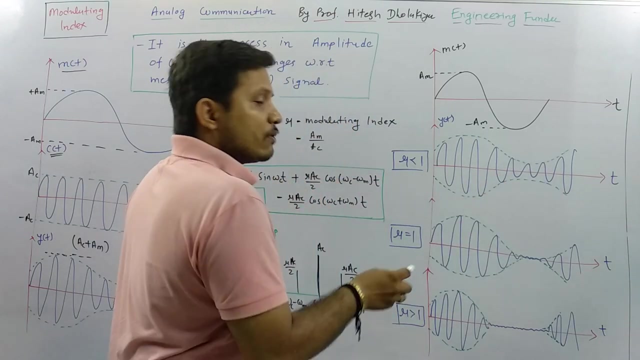 am is less than ac, then you will be finding somewhat envelope, is there? so here i have shown you that case where if modulating index that is lower than 1, then you will be finding somewhat signal, which is happening at minimum amplitude even. but in case of if you consider modulating index, 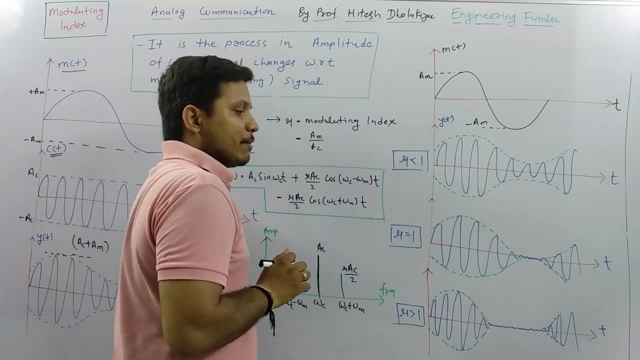 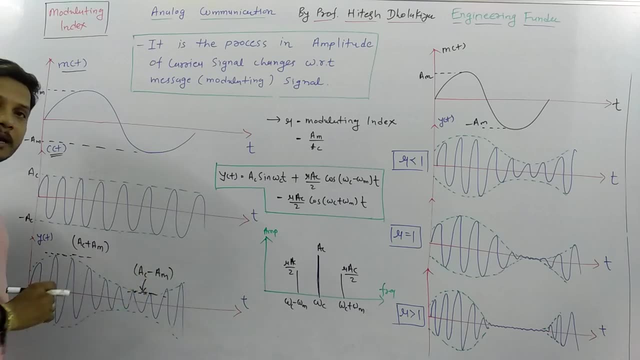 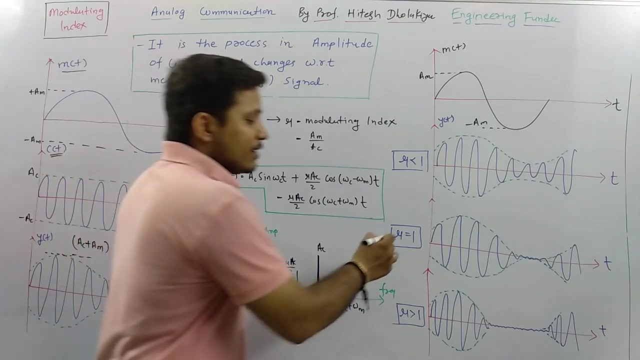 is equals to 1 means ac is equals to am. so what happens over here? signal is ac minus am, and if ac minus am- that is what ac and am are similar- in that case ac minus am will be 0. so you can see, if mu is equal to 0, then you will be finding somewhat signal which is: 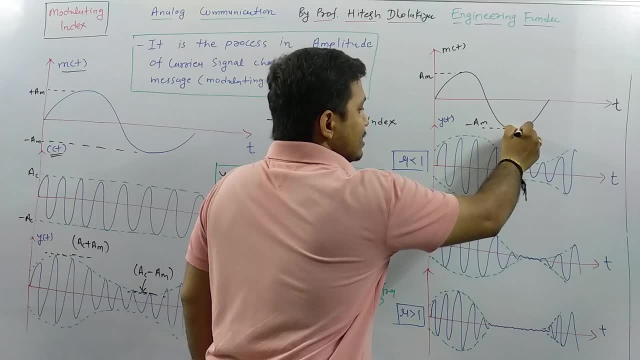 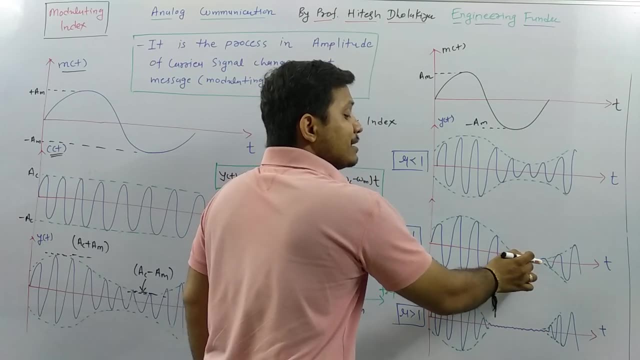 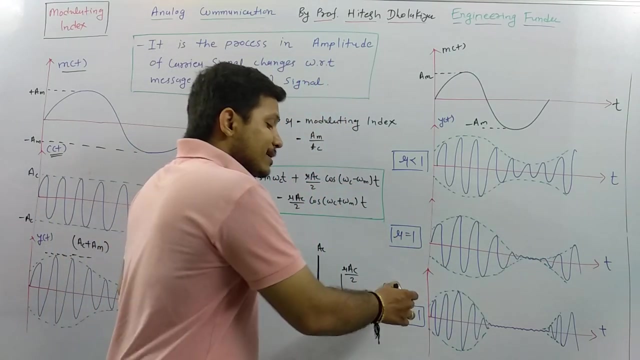 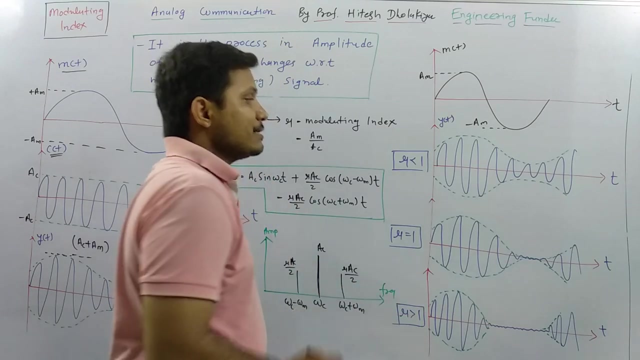 equal to 1. duas here: twist Понìn signals. output is 0. now if we consider modulating index, that is greater than 1. so if that signal is greater than 1, in that case your will be finding that distortion is happy. ok, what will? 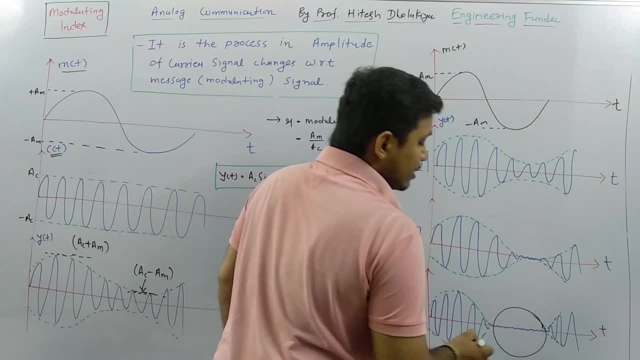 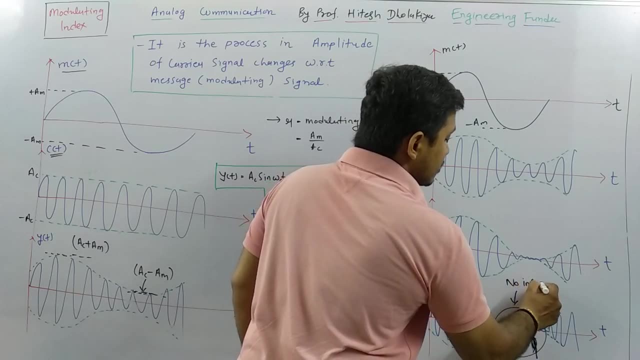 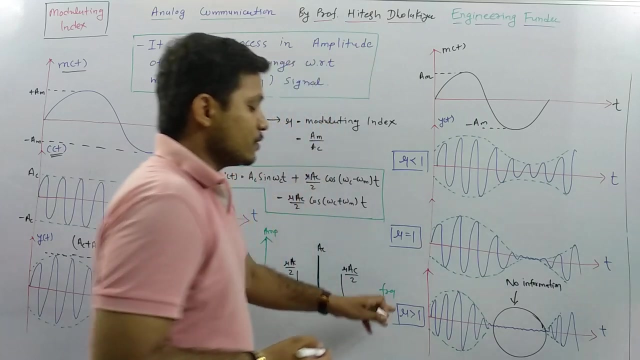 be happening. we are solely stating that can't fast forward happening. So this is what distortion? so here signal is getting lost. So no information. so here there is no information during this time period. So that is what the issue which will generate, as if you have modulating index that is greater than 1.. If modulating index 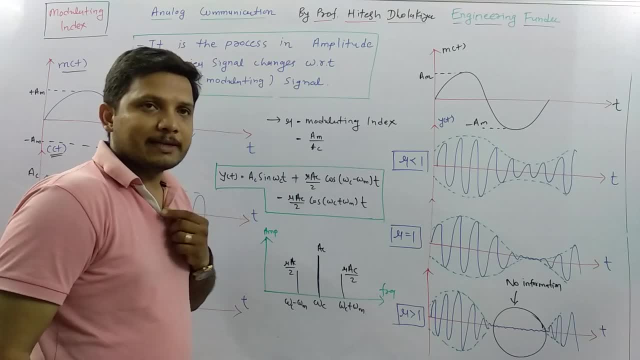 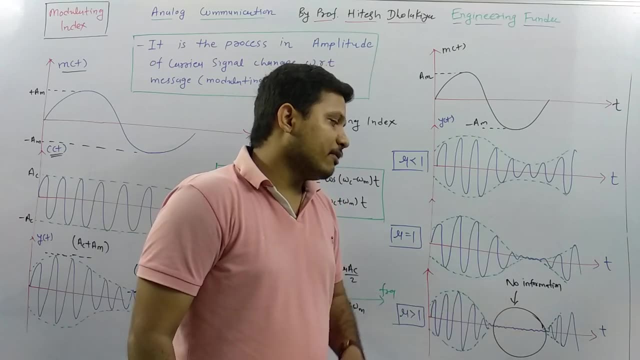 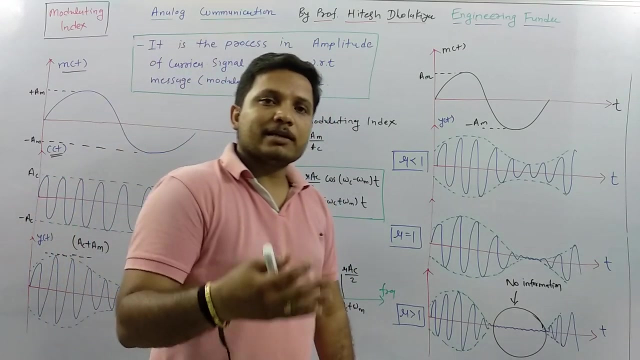 is greater than 1 means AM is greater than AC. So in that case there is a problem of distortion and where possibility of lost of information is possible. So that is what one issue Now see. in next session I will be solving examples based on amplitude modulation. So 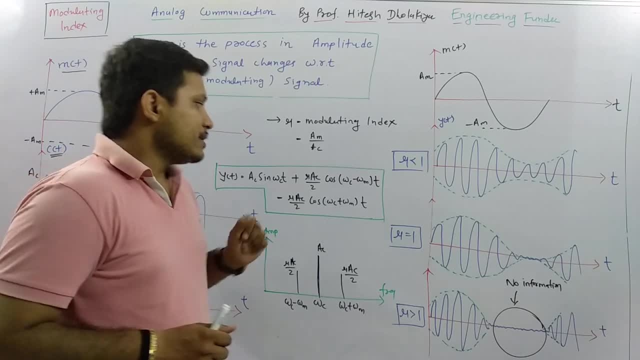 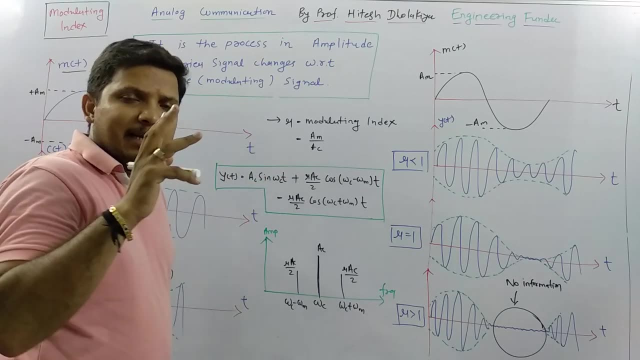 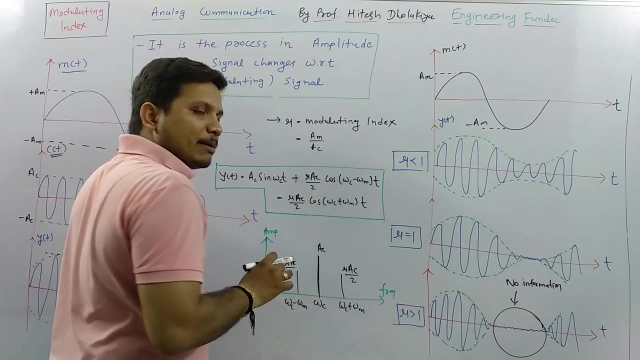 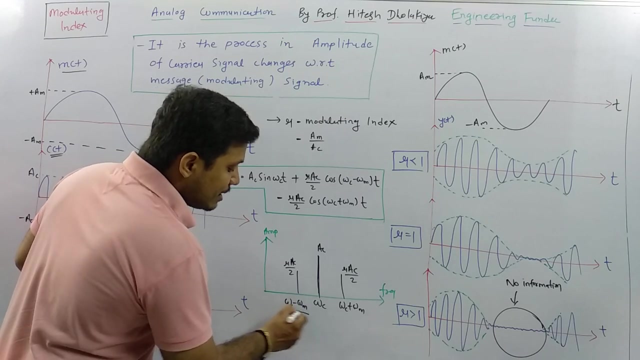 how many things that you need to keep in your mind. First is this basic equation. it should be clear to all. Like In AM signal, there are three frequency components: Carrier: omega c. lower sideband: omega c minus omega m. upper sideband: omega c plus omega m. So this is what lower sideband lsb. this. 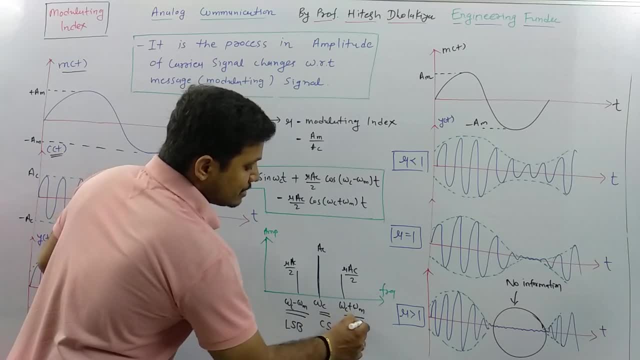 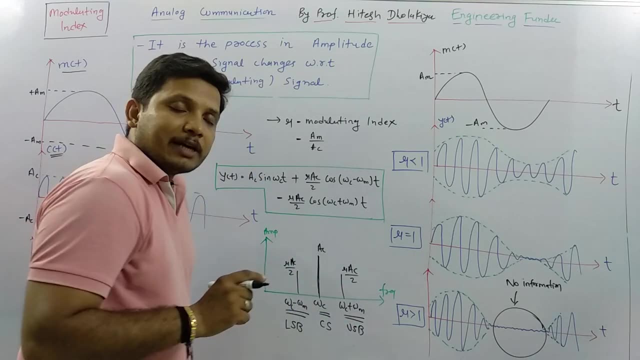 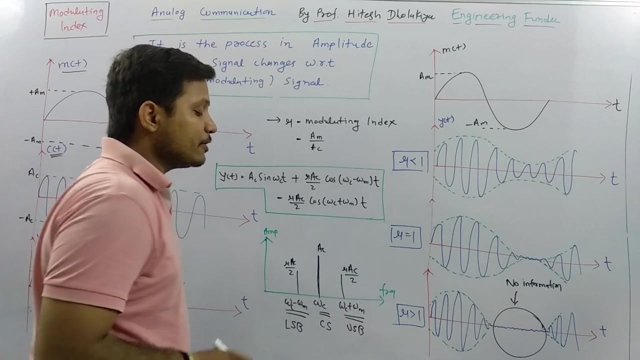 is what carrier signal- and this is upper sideband usb Carrier signal- is having. average frequency signal is havingнимal amplitude AC. lower sideband is having amplitude muAC by 2 and upper sideband is havingamplitude muAC by 2.. One more thing: modulated signal. that varies. 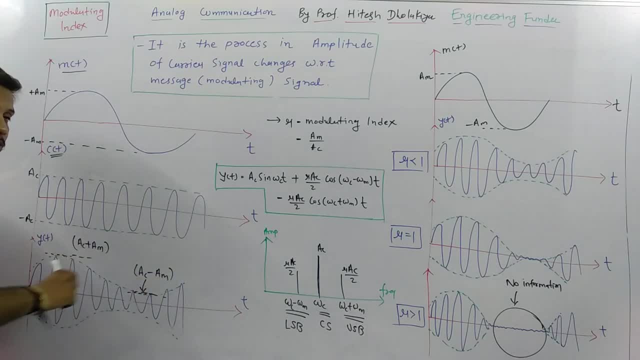 from maximum to minimum, where maximum is AC plus AM and minimum is AC minus AM. So maximum amplitdue, maximum amplitude, if I say you have an amplitude a, so the segunda is a, a plus milieu in the privacy, And a minimum amplitude of is m. So, comb, not have our ability that. 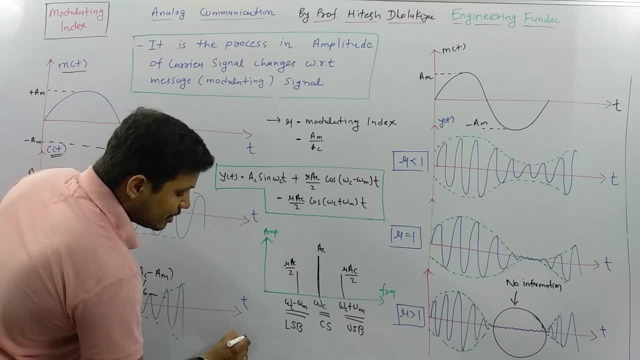 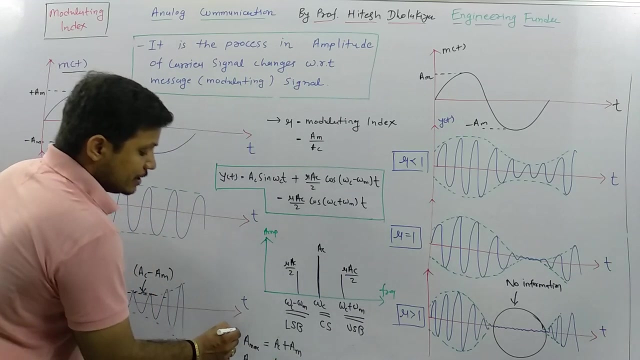 Nashville I. small amplitude in one input of the network. you have amo, north channelectomol, hip Titan. you have A max. So maximum amplitude is AC plus AM and minimum amplitude that is AC minus AM. So these many things that you need to keep in your mind to solve problems based on amplitude. 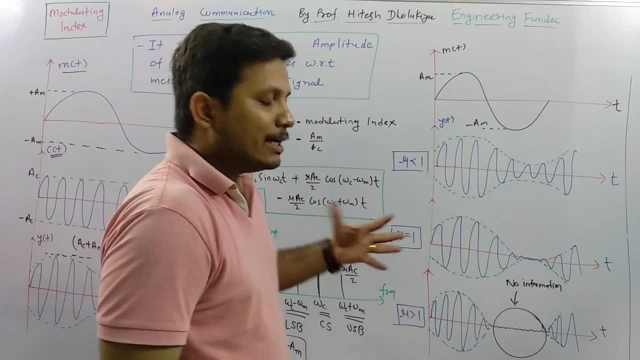 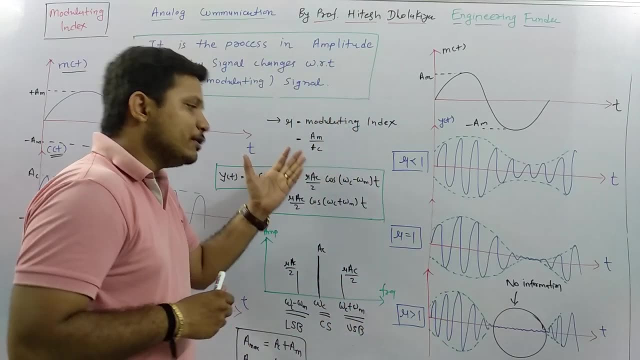 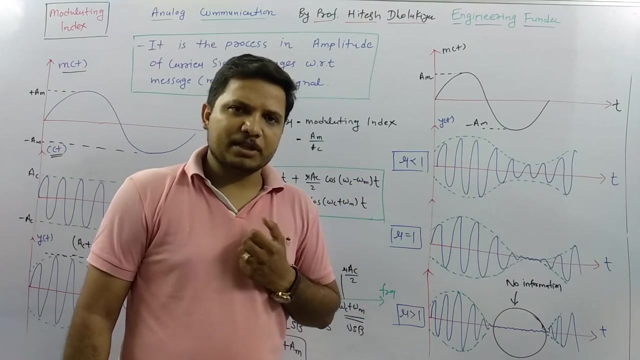 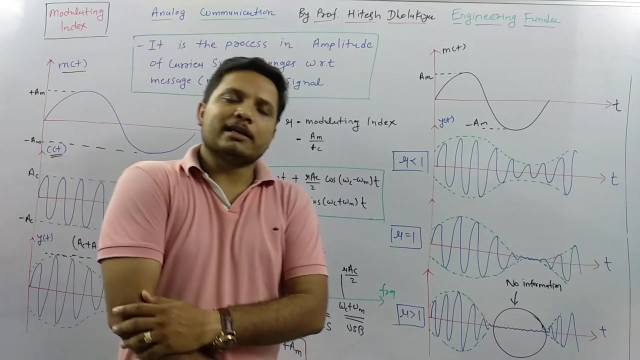 modulation. So modulating index plays very important role in amplitude modulation and these are the basic formulas that you need to remember to solve examples based on amplitude modulation. and that is even very important for gate examination where there could be a problem based on amplitude modulation. So one should know amplitude modulated signal.